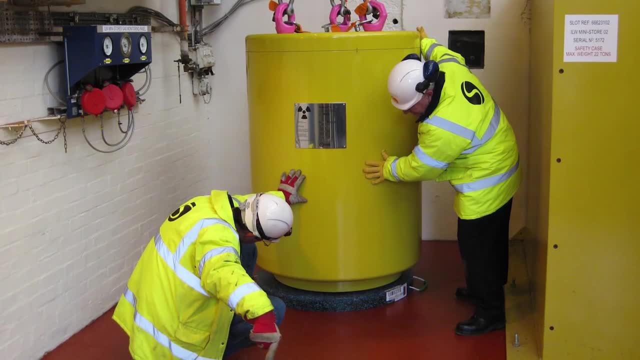 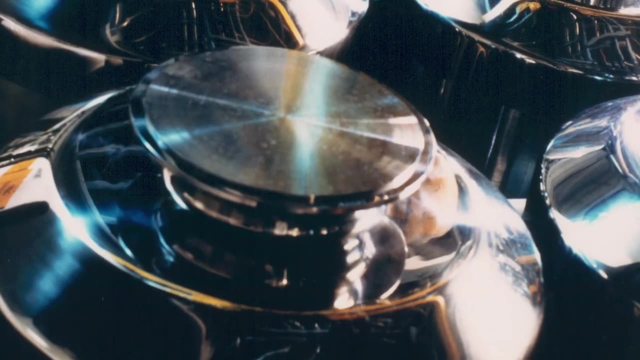 Above the certain threshold of radioactivity. the waste we have to treat is intermediate-level waste And there's a final category, which is high-level waste, And the only place in the UK that manages high-level waste is the Sellafield site. 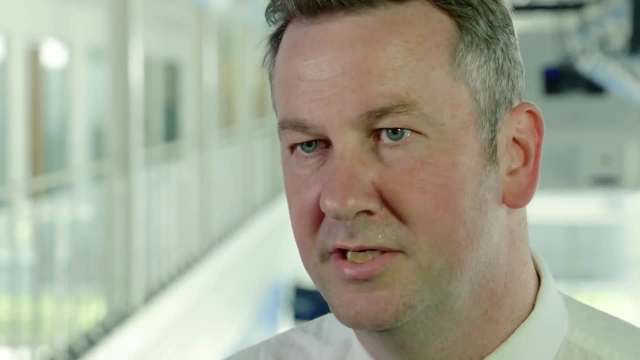 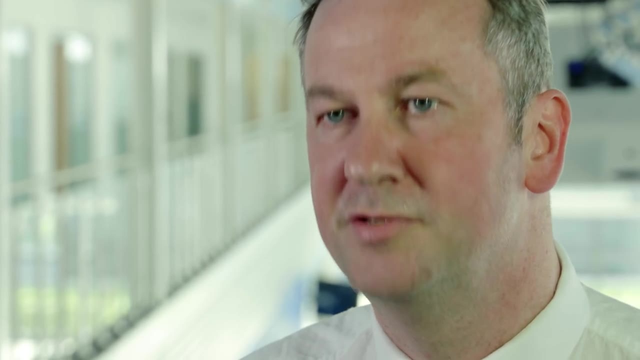 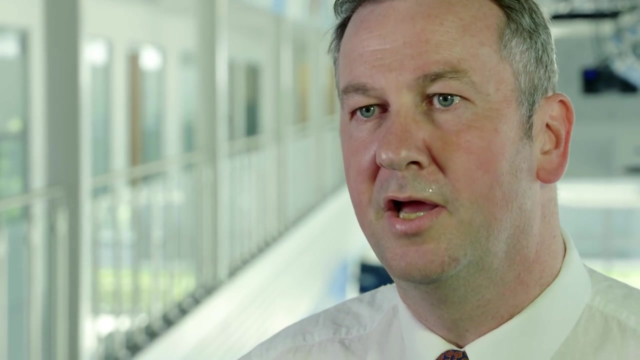 Waste management is a really important part of NDA's strategy. It's essential in delivering our mission In terms of site decommissioning and remediation. Without robust waste management routes in place, we cannot deliver our mission. NDA's role in terms of waste management is really to deliver strategic options. 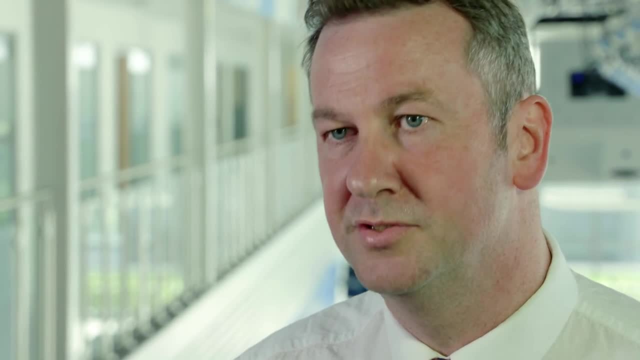 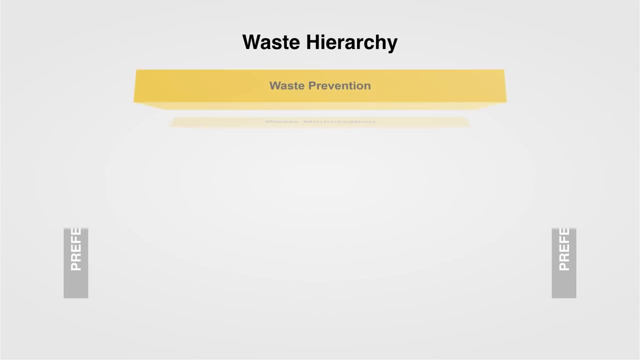 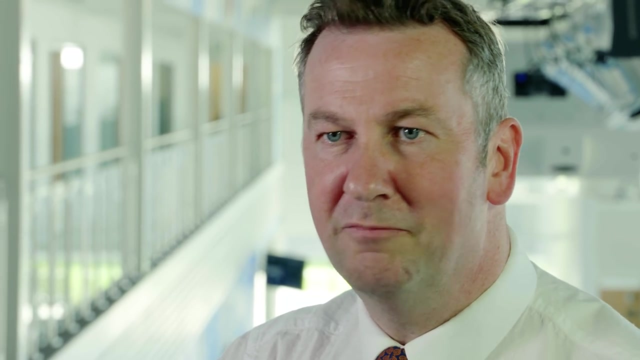 To provide a leadership role in developing strategic options that help to improve and optimise the waste management process across our estate. The waste hierarchy is an important tool for the NDA and the broader industry as well. It sets down a priority Of principles to help us deal effectively with our waste. 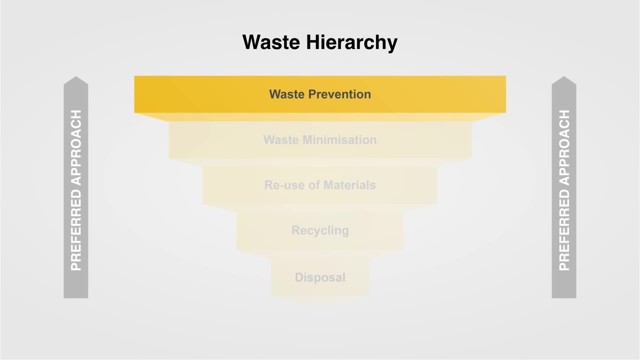 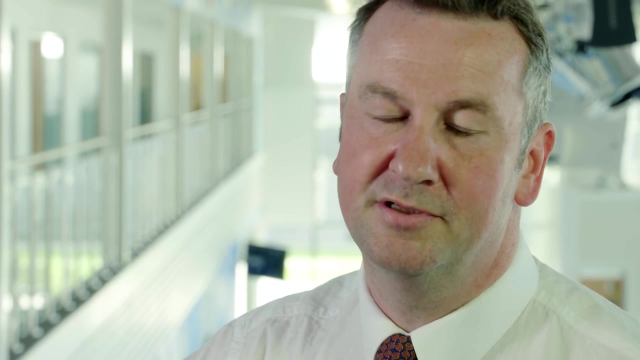 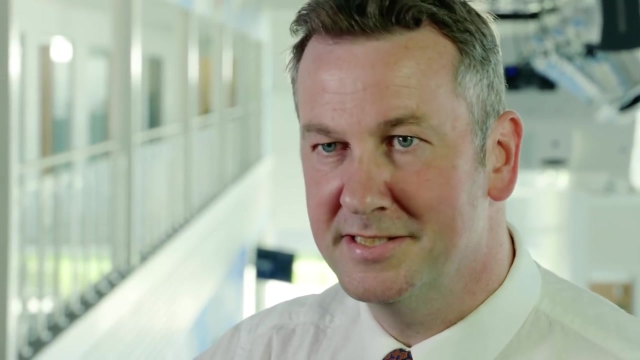 The first principle is waste prevention, And here is to consider the possibility of avoiding waste in the first place. If wastes are unavoidable, then how do you minimise those wastes? What technologies are available that allows us to minimise waste? And then it's about asking the question: could you extract value from the waste itself? 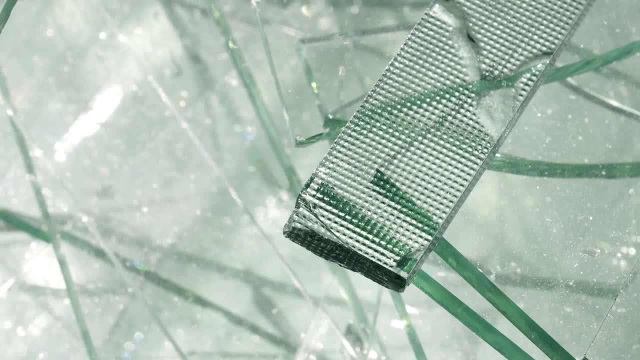 Even though there's a lot of data out there. Even though there's a lot of data out there, Even though there's a lot of data out there, Even though they've been deemed waste, there is often valuable materials in there, such as metals, for example. 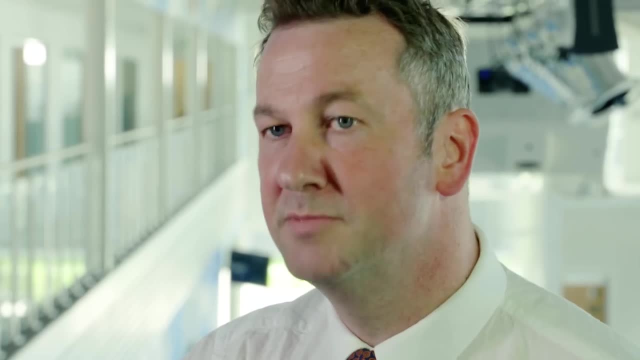 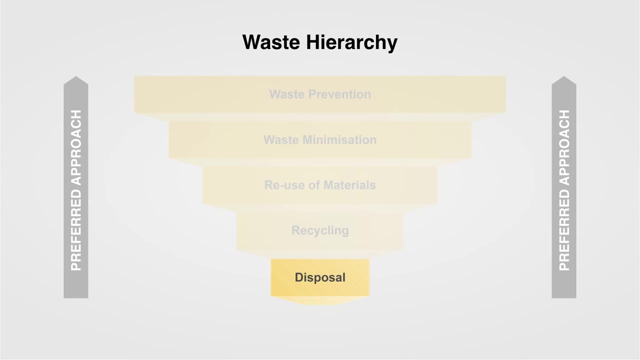 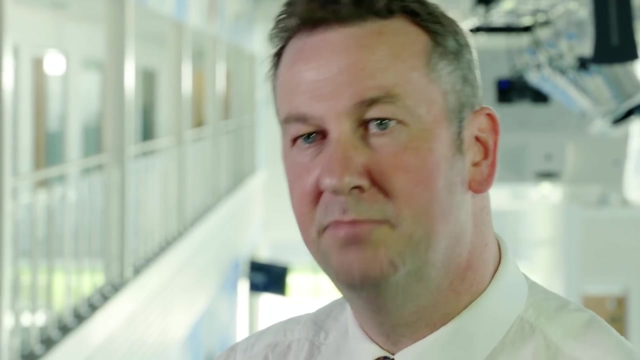 Could you look to reuse those materials? Could we treat them in such a way we can recycle it? And the last stage within the waste hierarchy is disposal. So often NDA and others will talk about eventual disposal, Recognising there's a series of steps in place before you have to dispose of those materials. 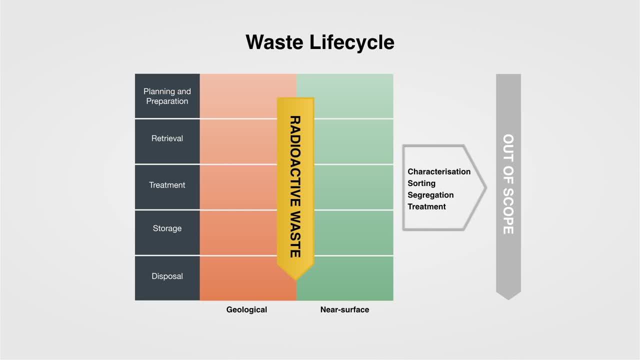 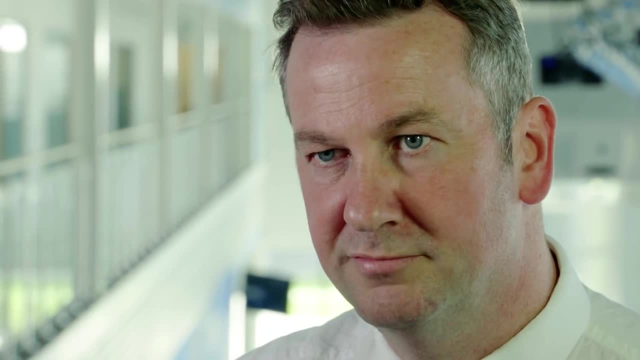 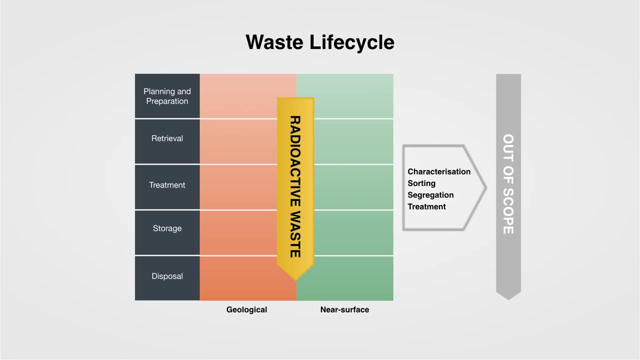 Waste management is not simply about getting rid of waste. It's about getting hold of some waste and finding the nearest disposal facility. It involves a number of steps, And the steps include waste retrievals, treatment, storage, if applicable, and then disposal. 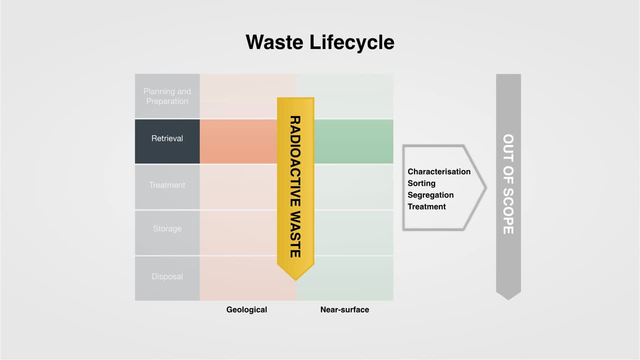 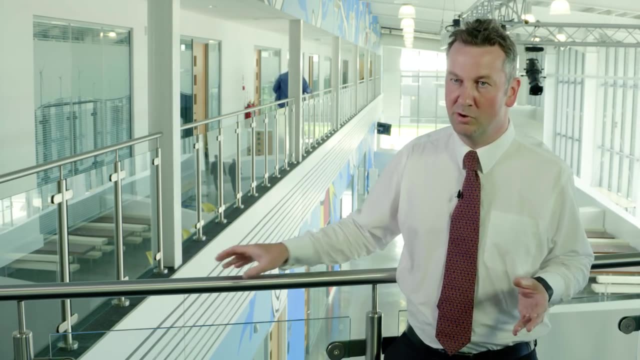 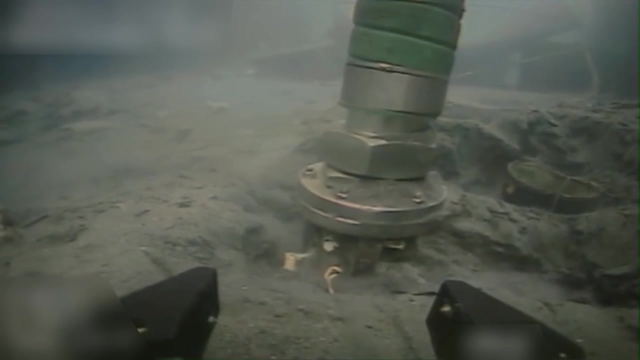 Waste retrievals is a key area because by retrieving the waste you're then allowing the next step in the waste management lifecycle to proceed. So waste retrievals is an ongoing programme of activity across the whole of the NDA state. Examples are on Sellafield site, where we're making progress. 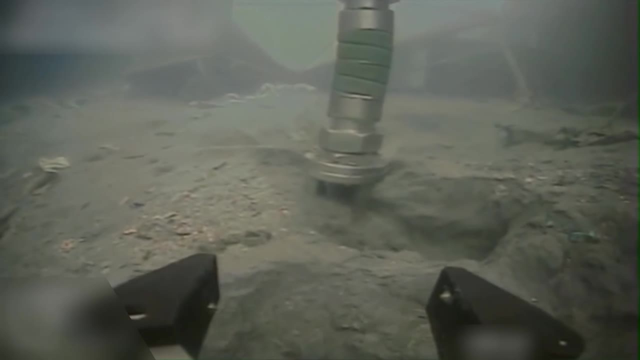 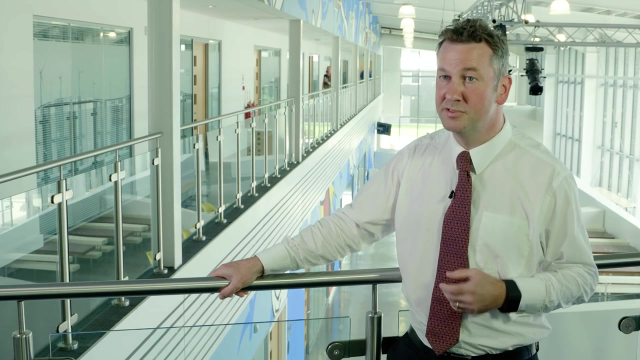 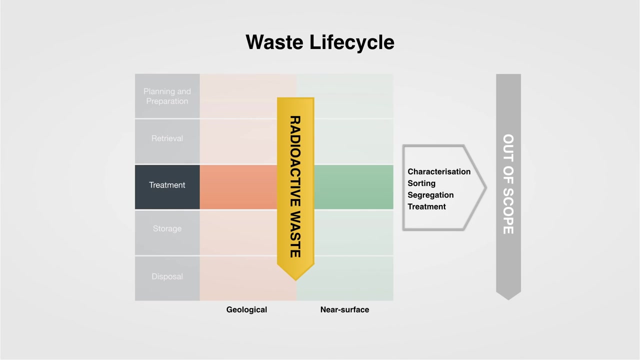 and retrieving radioactive sludges from our legacy facilities. Our process has just begun. Other areas are on our Magnox sites where we are retrieving solid waste from bunkers on those sites. For example is Hunterston. Waste treatment and supporting the waste hierarchy is a really important area for us. 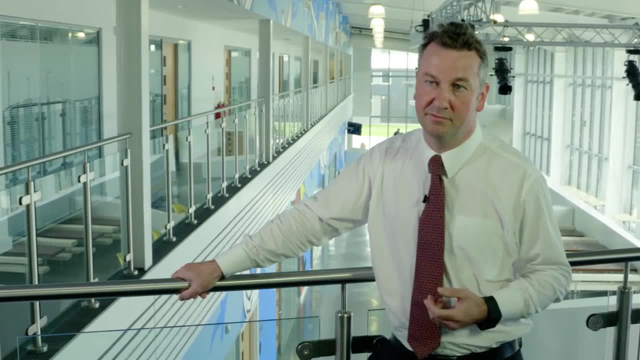 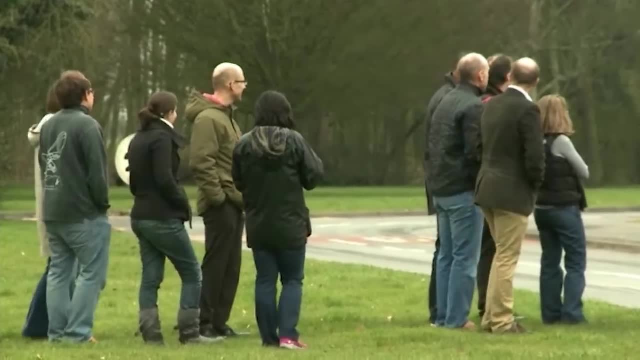 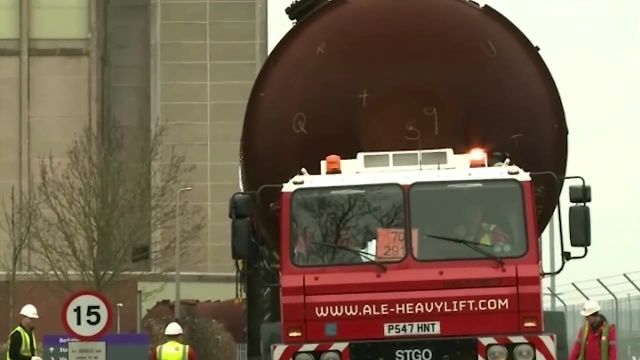 We've got clear evidence of how this is making a difference. For example, at Barclay we had some very large boilers that, because of treatment, were able to recycle the majority of that material back into the industry, where only a fraction of that total material ended up in our low-level waste repository. 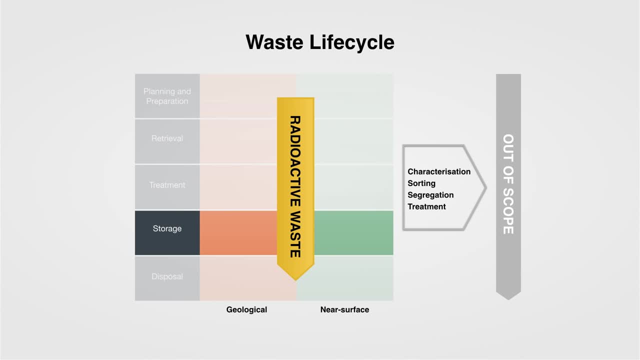 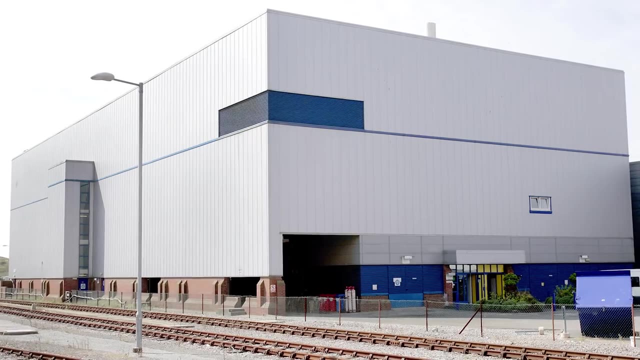 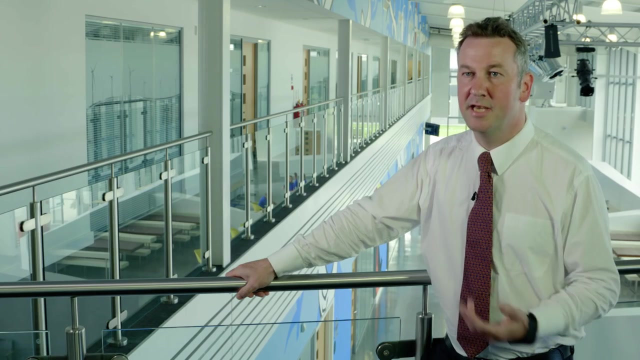 Waste storage in support of the high-activity waste strategy is really important. In the UK we have no available disposal route for high-activity waste, So storage needs to cover a period of a decade And in support of that, the NDA delivered industry guidance which provides detail and information. 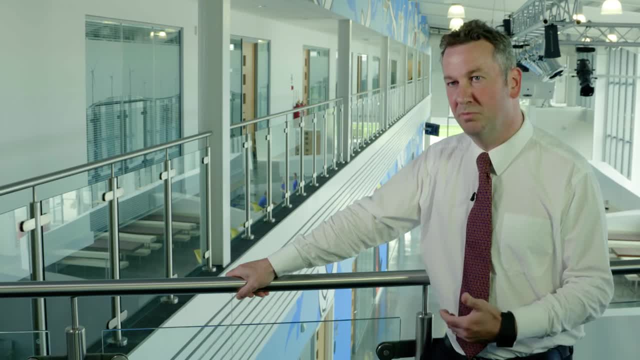 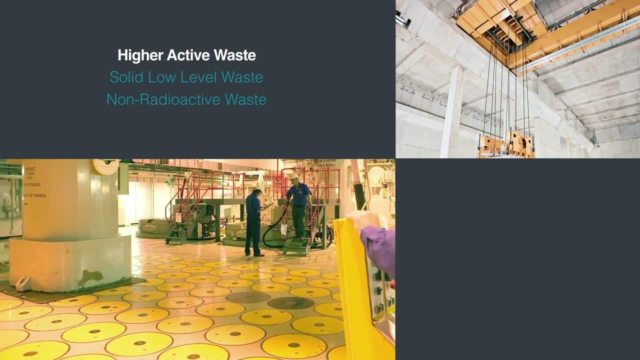 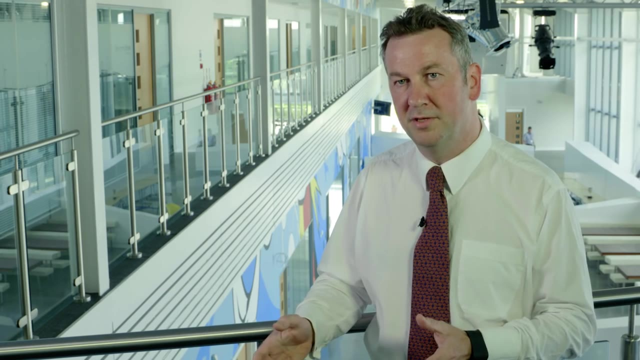 and also principles in support of how best to support the storage strategy. Currently, our strategies cover a number of areas: high-activity waste strategy, solid low-level waste strategy, non-radioactive waste strategy and discharges as well. Moving forward, our aim is to have a more integrated approach. 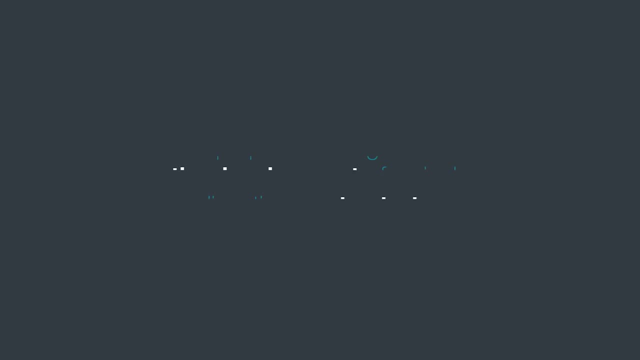 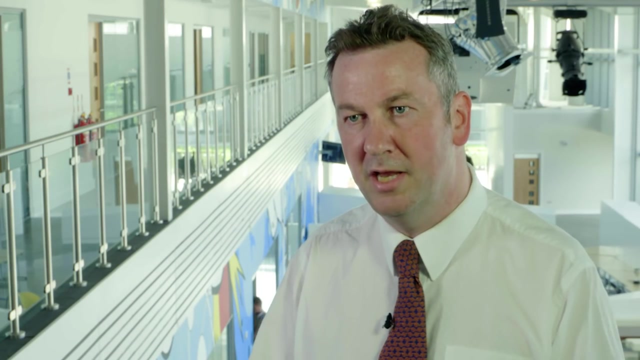 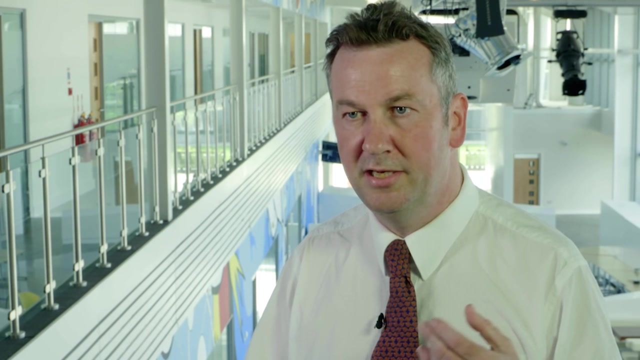 as in the title of our theme area, which is Integrated Waste Management. What is the role of the NDA? Rather than having separate, individual strategies in the radioactive waste area is to have a single radioactive waste strategy that clearly investigates and looks at those boundary areas between, for example, 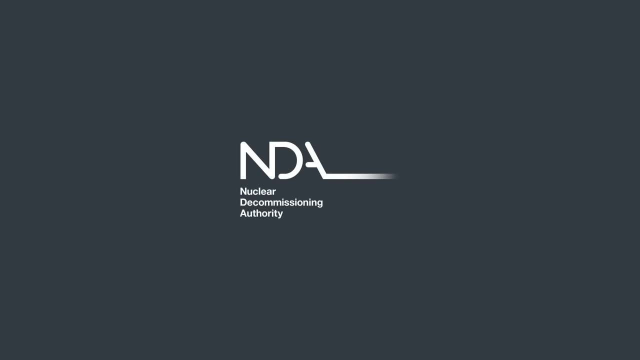 intermediate-level waste and low-level waste. What is the role of the NDA in the future? To find out more, visit us at ndagov.